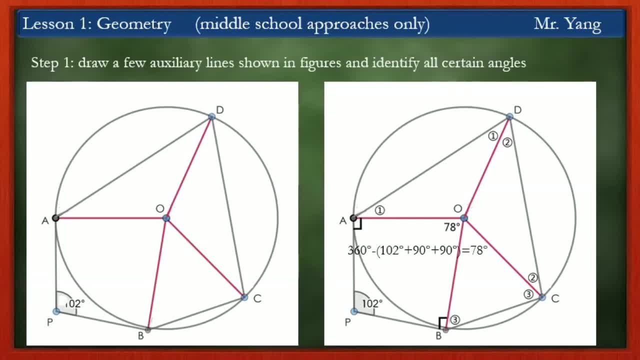 On the left hand of your CV have drawn four red auxiliary lines. On the right hand of your CV have drawn four red auxiliary lines. On the left hand of your CV have drawn four red auxiliary lines. I identified all certain angles In quadrilateral APBO. we have worked out the angle aob, which is 78 degrees. 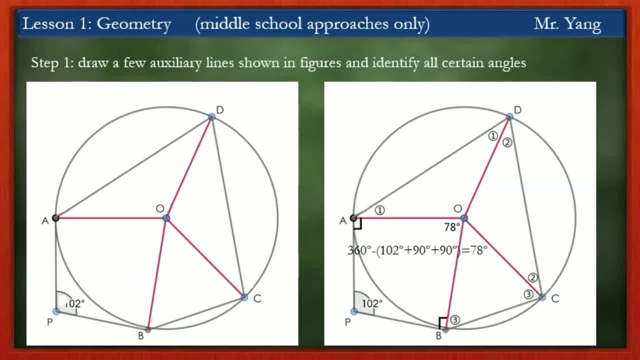 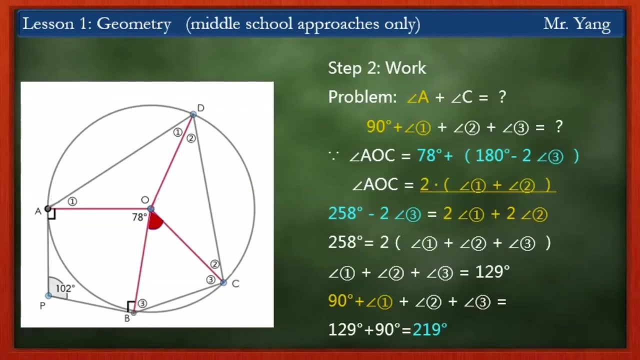 The three triangles aod, doc and cob are all isosceles triangles. Therefore, we have three pairs of equal angles: a pair of angles ones, a pair of angles twos and a pair of angles threes. that's all we have now. let's move to step two. our problem is we. 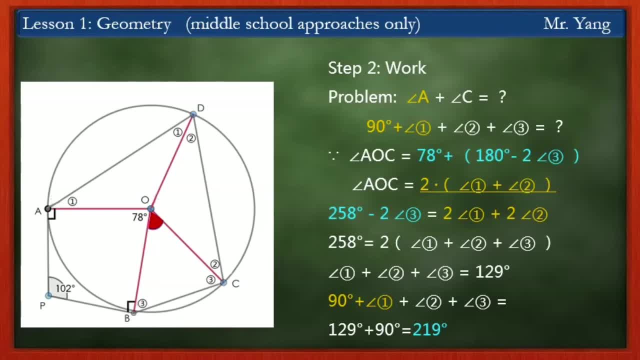 have to work out sum of angle A and C. right now we substitute angle A with 90 degrees and angle one. we substitute angle C with angle two and angles three, because we know angle A or C equals 78 degrees and difference of 180 degrees minus two times angle three. at the same time, we know angle A or C is called. 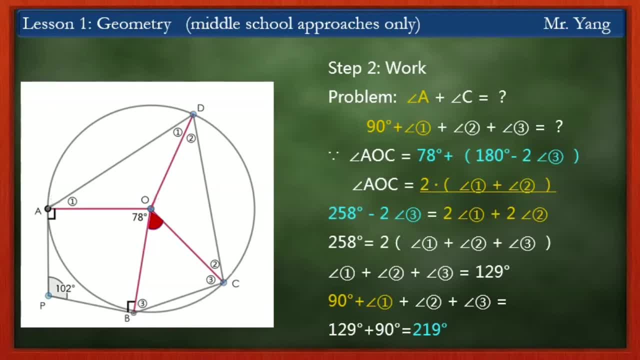 central angle or radial angle right, which is two times of angle of circumference, circumference, angle of circumference, ADC. therefore, we have: angle A or C equals two times sum of angle one and angle two, which is very important. if you know the relationship between central angle and angle of circumference. now, this is the key to the problem. now let's simplify. 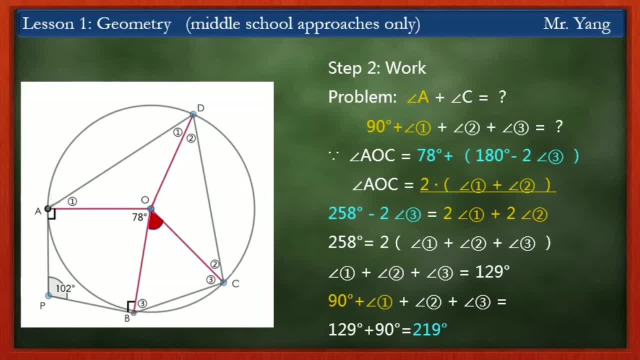 them. 258 degrees minus two times angle three equals two times angle one and two times angle two. 258 degrees equals two times of sum of angles one and two and three. now we work out sum of angles one and two and three, which is 129 degrees. finally, we worked out the solution, which is 219 degrees if